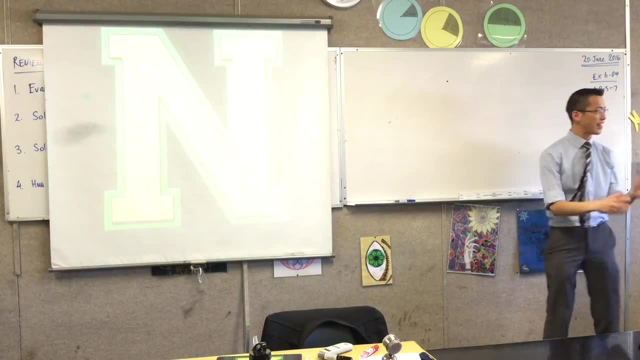 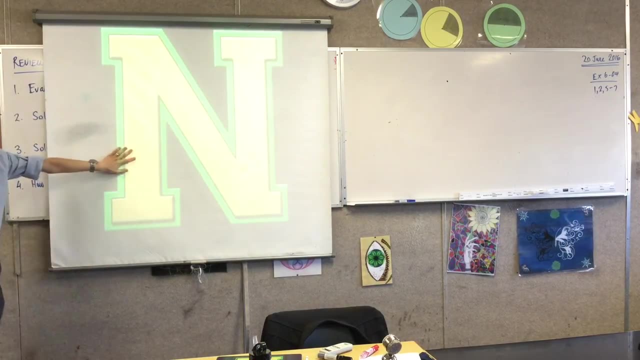 Now here is a picture. Now, I don't want you to say anything, I just want you to think with me. okay, Like I said, don't shout it out, Just answer up here. The question I want to give you is: is this symmetrical? 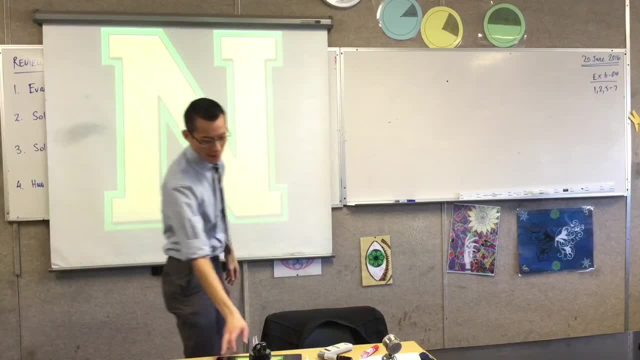 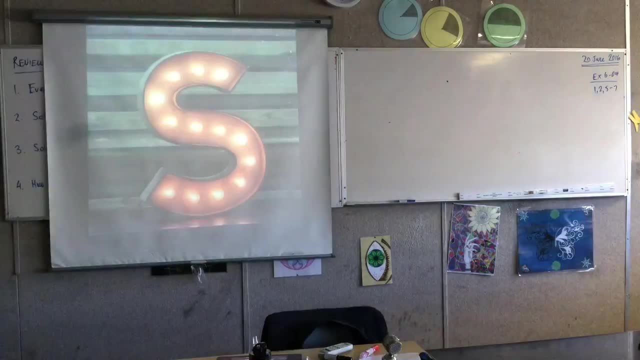 Have a think about it. Have a think: Is it symmetrical? How about this shape? Is that shape? Let me get the lights for you, That might make it a bit easier. Is this shape? Is this shape symmetrical? Cool? 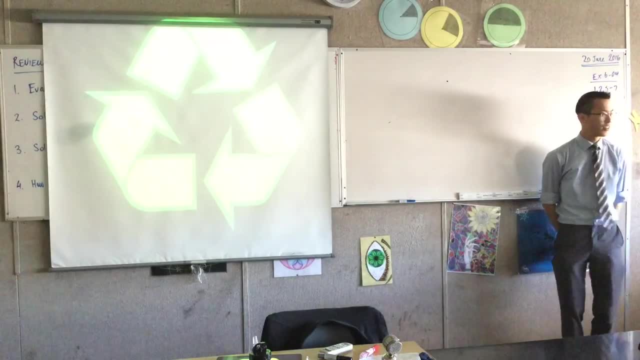 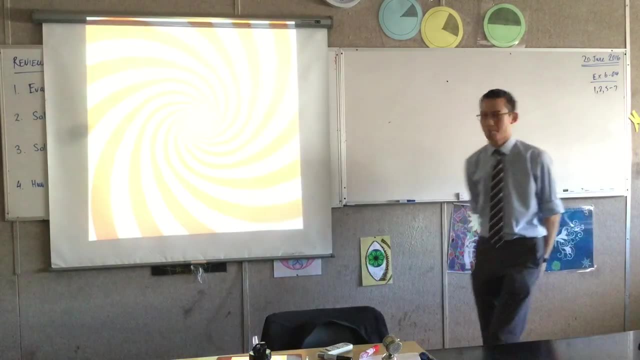 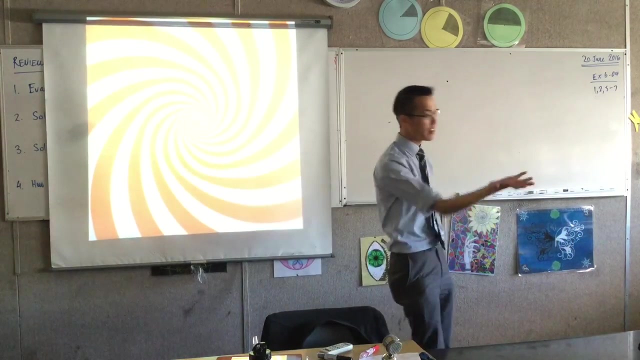 What about this one? Not symmetrical? You don't think so? No, Yes, No. What about this one? Yes, It's not even a shape. Okay, so let's Well. I mean, it's a pattern, It's an image, okay. 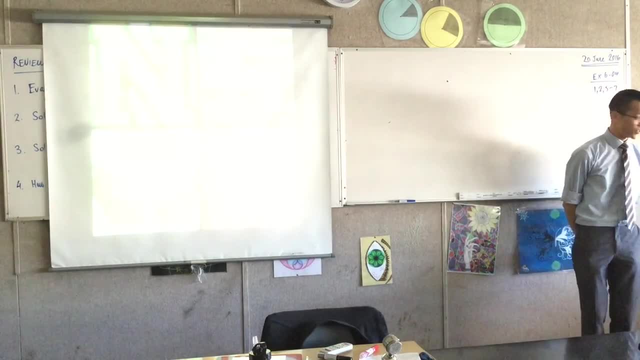 So let's think about these right Now, when you look at all these images together and, in fact, this time now Leave space for a heading. I'll tell you what it is in a second. This time I do actually. 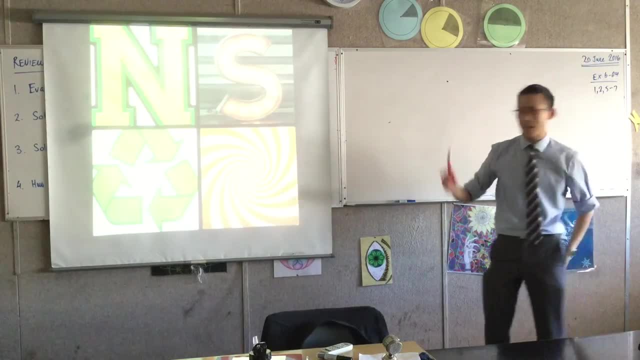 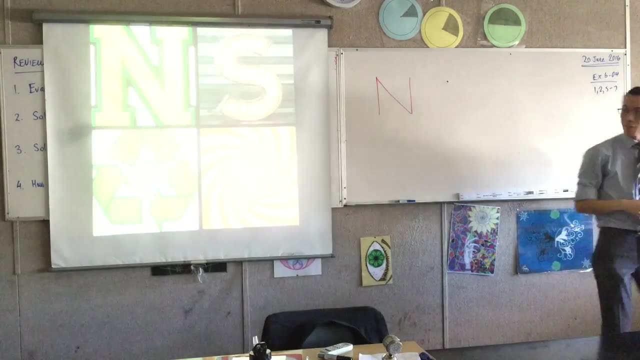 I actually want you to draw one of these with me. Let's do the letter M. N's are easy, Okay, and after all, we are 7N If you. If you draw an N for me, Draw an N for me. 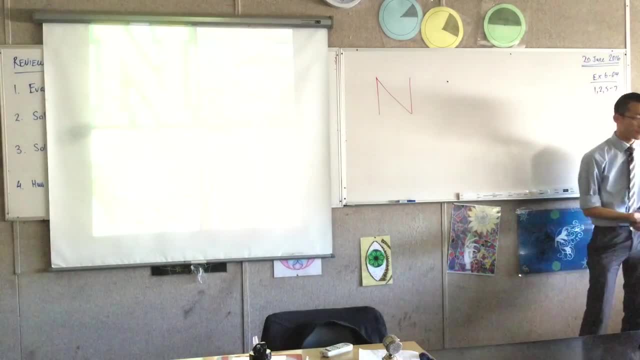 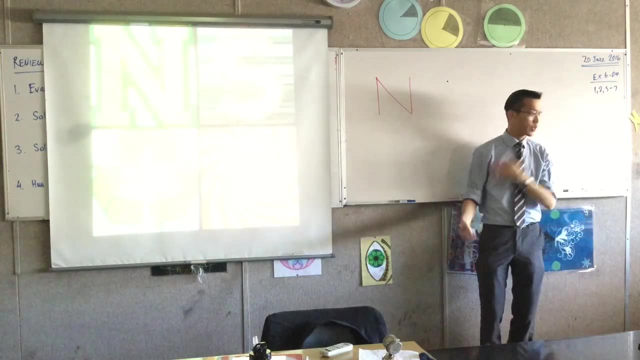 When we ask this question of is it symmetrical or not? okay, The way you know, Do you remember? I tried with the rectangle- Is you want to draw a line through it, which we call the axis, so that if you reflect across there? 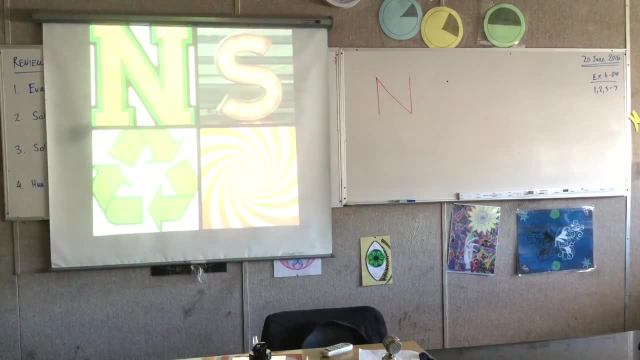 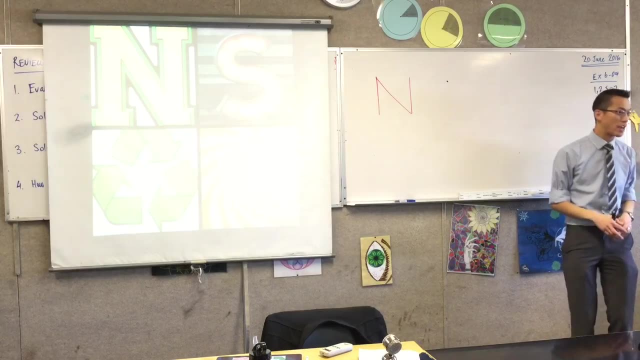 it's the same thing on both sides. remember that. Now let me just, So we can all see it, Let me see what happens. Where would you like me to put a line, What kind of line would you like me to draw, and where should it go through? 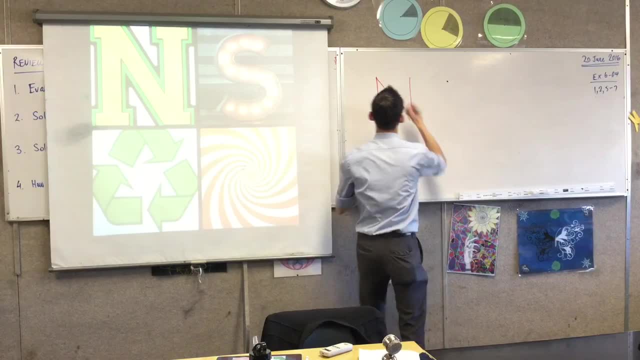 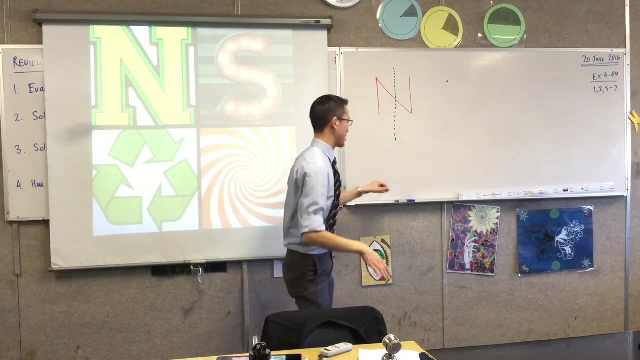 Yeah, right there. Okay, so I could draw a vertical line like this. Maybe you want to draw this with me. Okay, Now you might remember when we did our kind of little exercises and experiments on reflection. right, If I were to fold a piece of paper over? 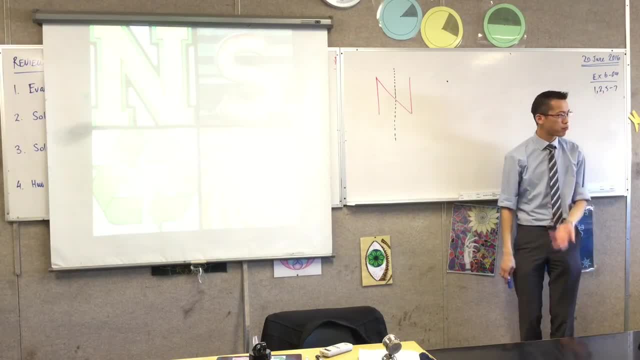 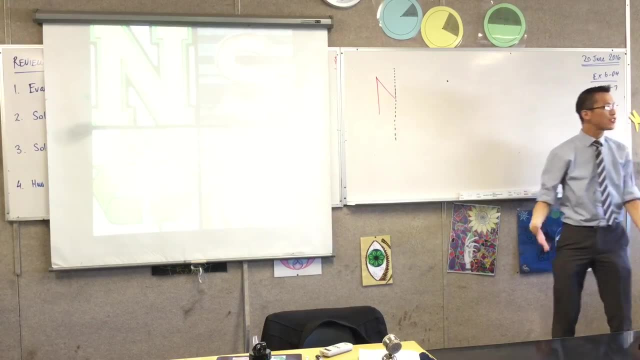 and try to reflect across this shape I kind of run into, I run into a problem, okay. So for instance, I'm going to rub off this side, So that leaves only one half of it When I do my reflection across what happens. 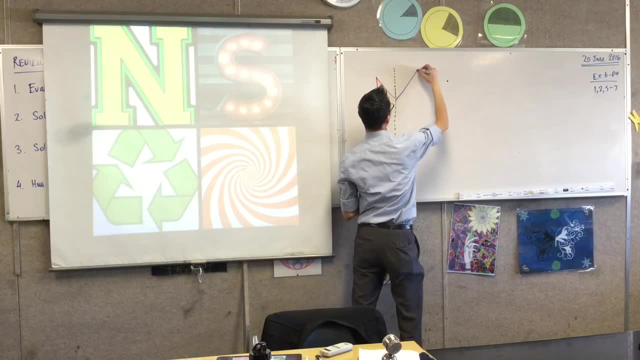 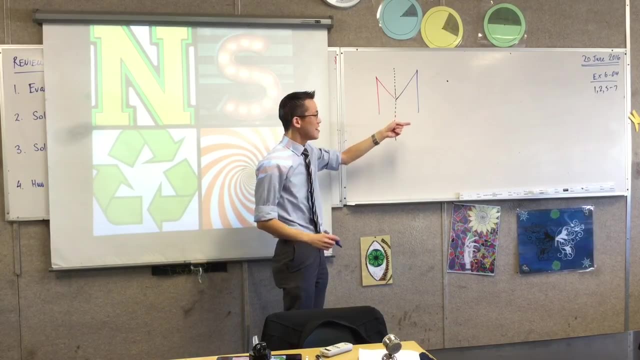 It makes like a weird M. Yeah, that's exactly right. This, this shape, has reflectional symmetry, But that's not the N I started with, is it right? So the N is not reflectionally symmetrical, Neither is the S. 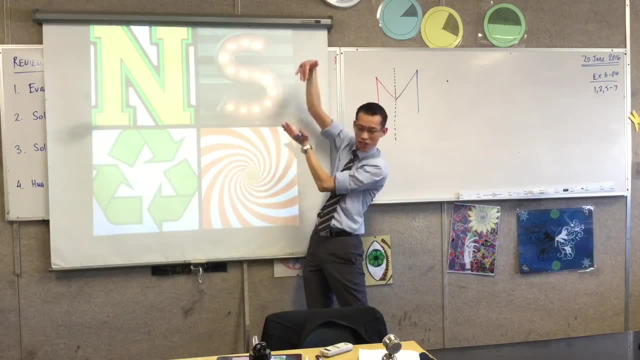 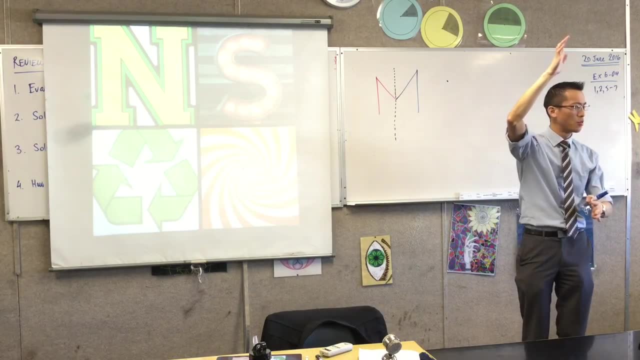 You can't find a line that you can draw through this. It doesn't matter which kind of way you go, Or the recycling logo, Or this weirdo-looking spiral, But I think we all agree, Because a lot of you said Yeah. 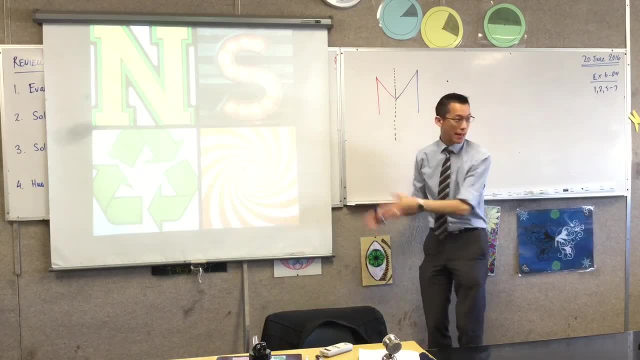 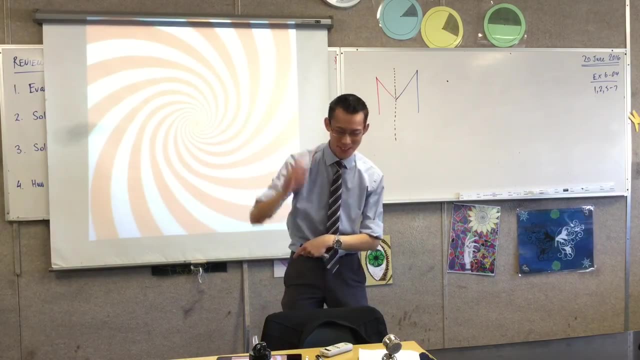 Wait, You know, there's something about this. There's something about this that is symmetrical. Now, I think Fatima said it. What did you say when you went to the S? It's a Before the spiral. you said something about this shape. 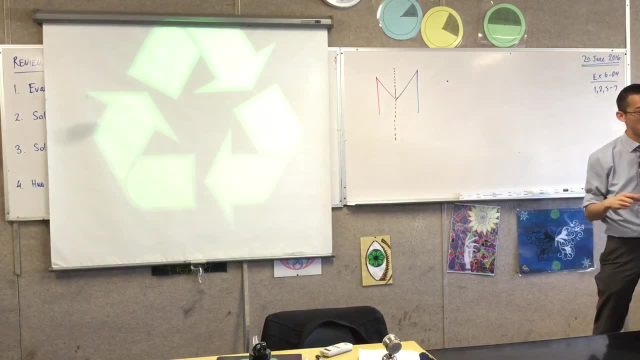 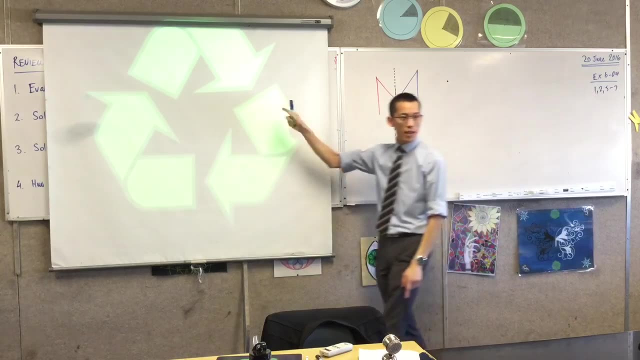 Do you remember Something about another way? I could transform this shape? You could turn it, I could turn, I could rotate it Instead of flipping or reflecting it. And do you notice, If you have a look at this, If I grabbed it? 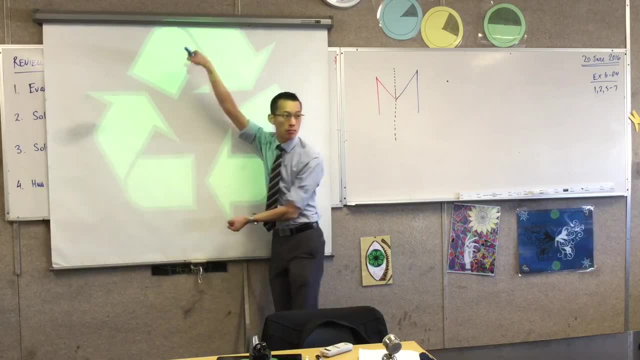 Took this side here And put it at the top Right, It would still be the same shape. And in fact, not only could I do it once, I could do it a second time, And I'd still get the same shape. 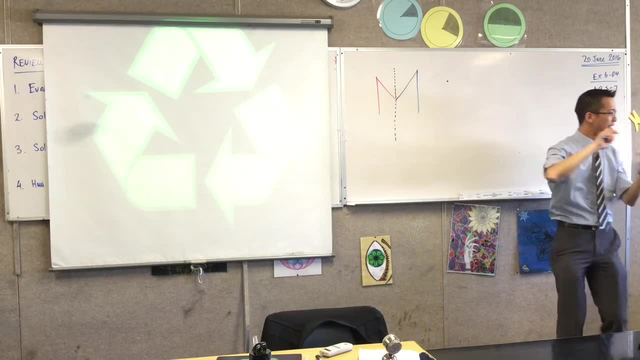 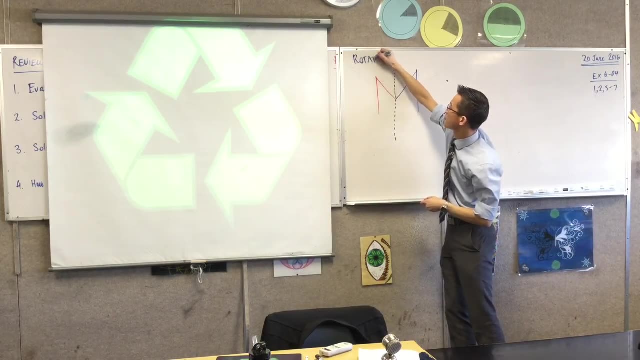 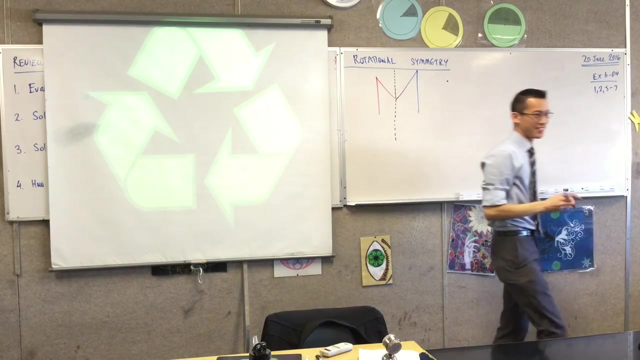 So what you find is that I can reflect to get symmetry, But I can also rotate to get symmetry, And that's the heading of today: Rotational symmetry. I said that you could rotate it to the S as well. Yes, very good. 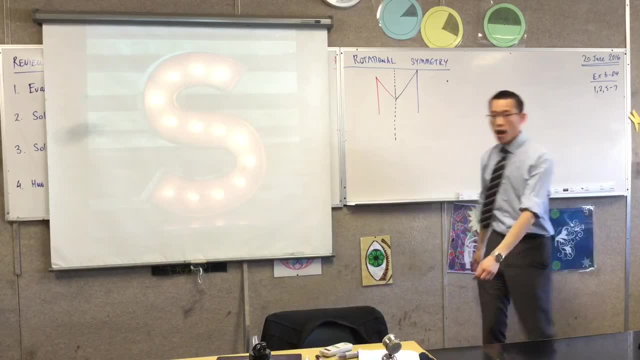 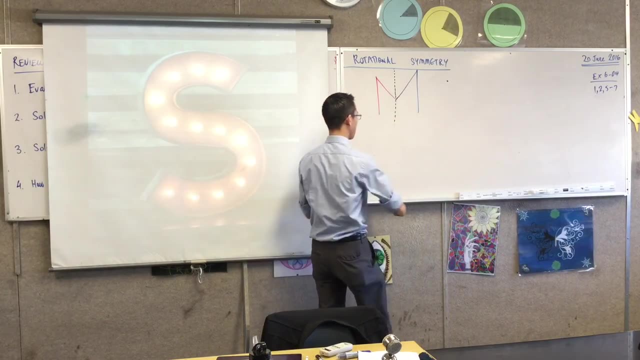 In fact, all the shapes that I showed you. All the shapes I showed you, Instead of reflecting across a line, Redraw your N again. Can you do that for me? If you redraw your N, You don't want a line. 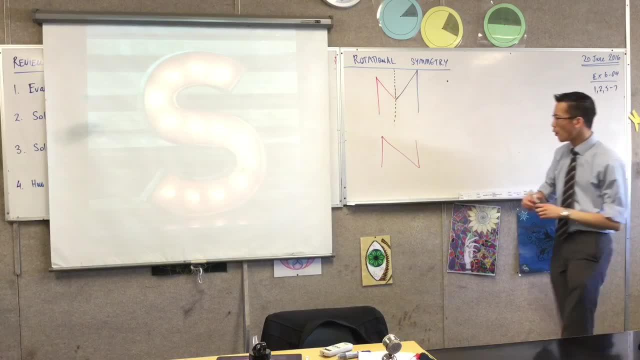 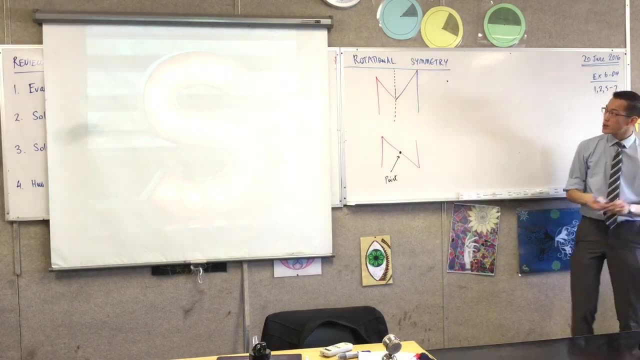 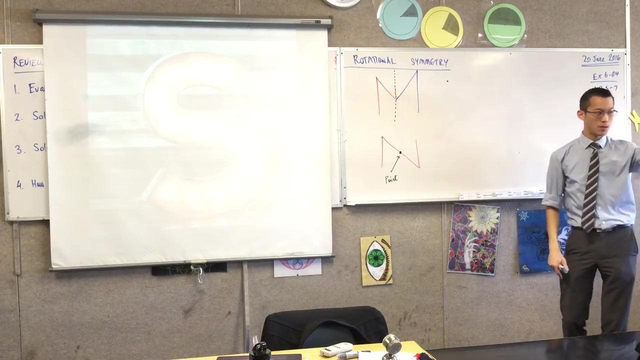 You don't want a line. In fact, what you want is a point Now, because this N here, The N that I drew by accident, This is reflection symmetry, But it's across a line, So that's why you might remember me as Lordy called it. 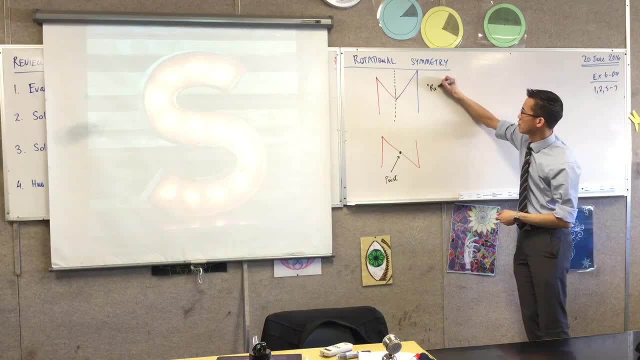 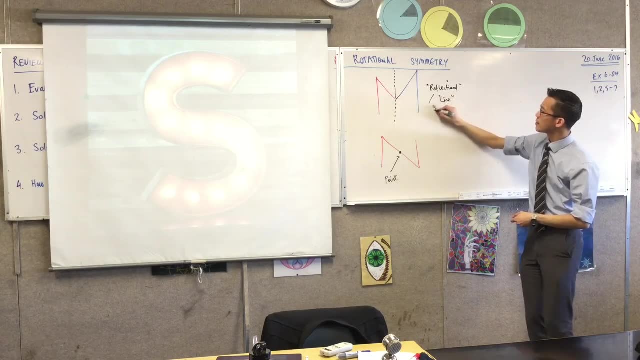 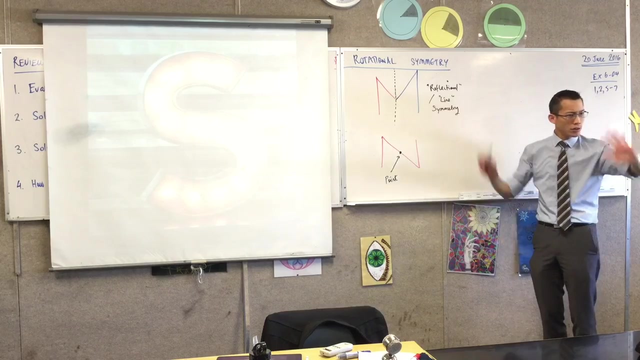 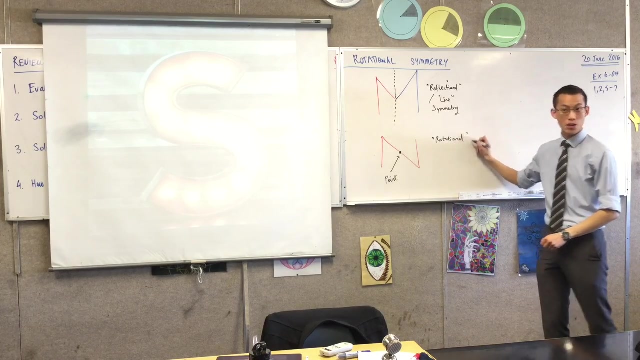 Line symmetry. So this is reflection Or line symmetry, Whereas this guy here It's not about a line at all. No lines required, It's just a point. Okay, So we call this rotational symmetry Because you have to spin it around. 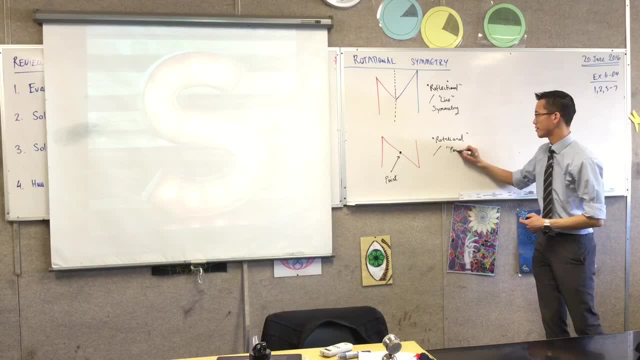 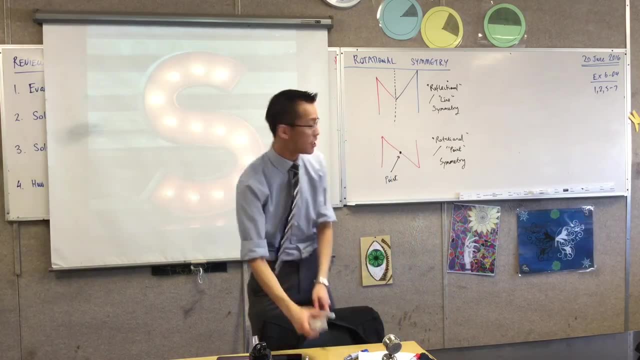 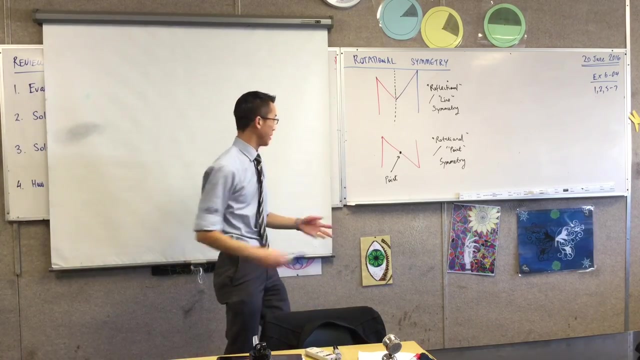 Or because it's about a point, We also call it point symmetry. Now, all of these are different kinds of symmetry And they're all important. Okay, Symmetry. in fact, You might remember when I talked about geometry. What does metri mean? 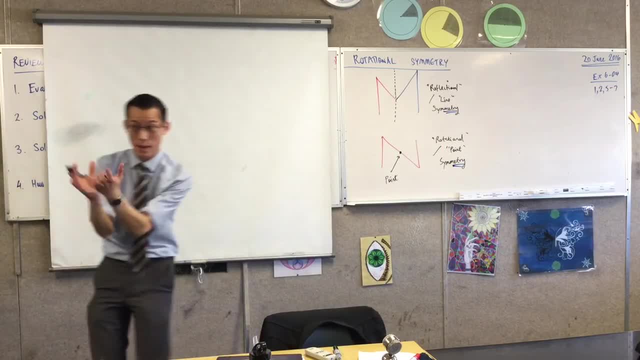 What's that about Meter? It has to do with meter. It's got the same root word as meter. It has to do with measurement, Right? Do you remember? like the metric system? That kind of thing, That's classic. Does anyone know? 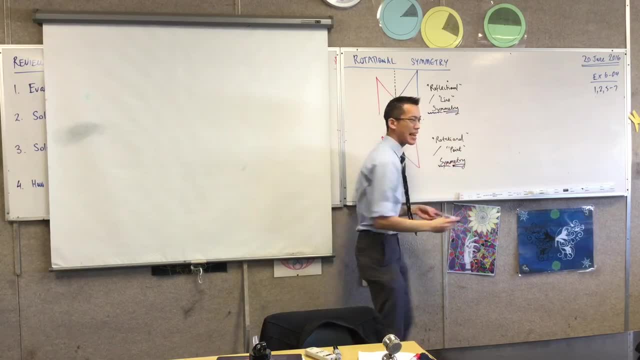 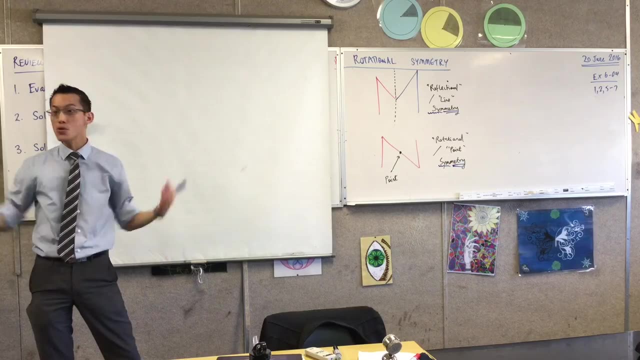 Does anyone know what happens, What it means, when you have this sym, This S-Y-M prefix on the front of a word? There are words you know: Symmetrical. Well, we have symmetrical. Can anyone think of any other ones? There's a musical word that starts with sym. 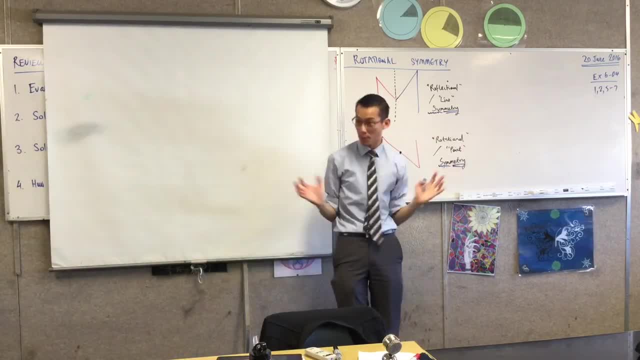 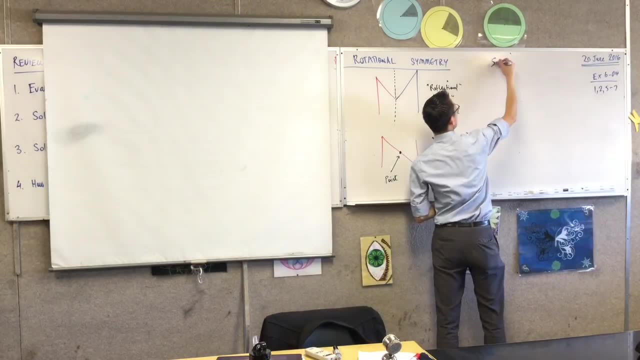 Symphony. You've got a symphony Where you've got a whole bunch of people And they play Sym, sym, That's just a name. You've got symphony. You might want to write this at the top. You might also have simultaneous. 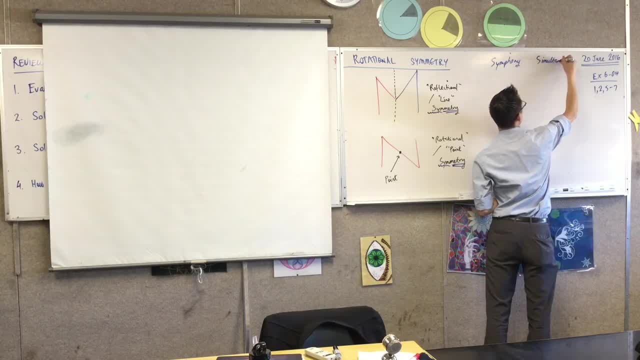 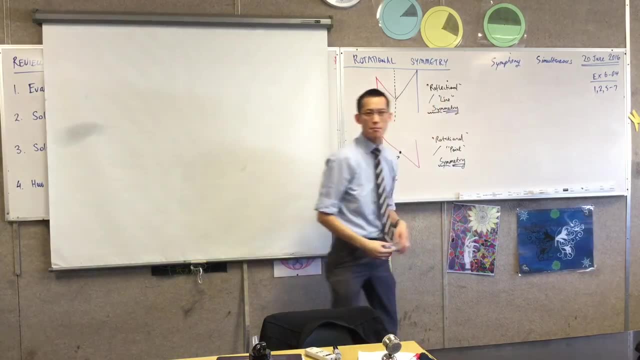 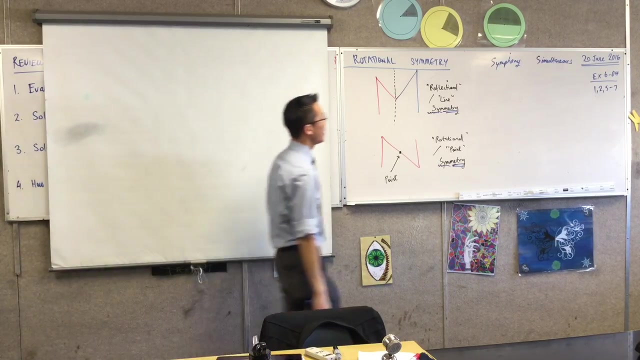 Right. What these things are is an agreement. That's what sym means Agreement. So symphony is agreement in sound Right, Phony as in like telephone Okay, And agreement in sound. This is an agreement in time, when things are happening simultaneously. 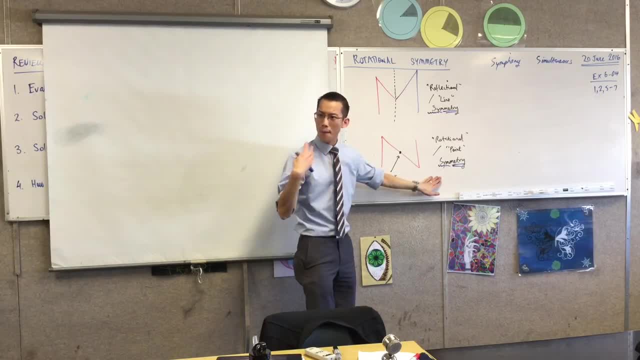 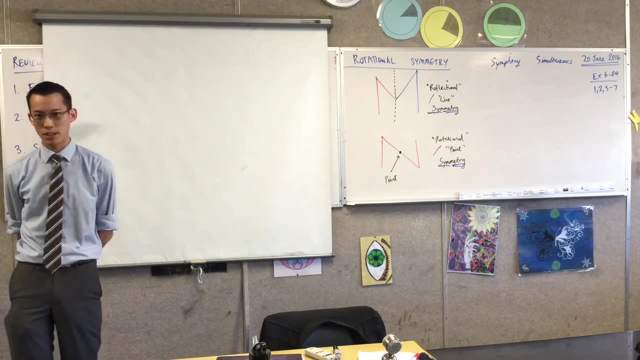 And this is an agreement in time, This is an agreement in measurements. Right, It's not the same, but it's got the same idea. The principle underneath is very, very similar. Okay, Now, last thing before I show you something really cool. 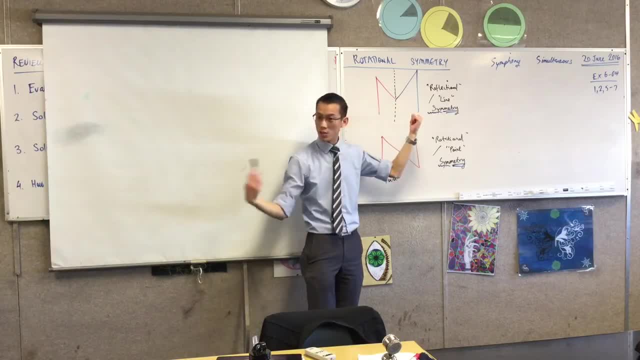 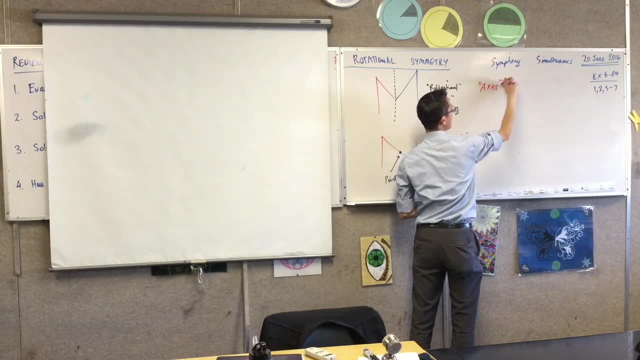 I'm so excited to show you this Right? Do you remember Like we looked at the square? If you have a reflection of symmetry, then it has. the more reflection of symmetrical it is, the more axes of symmetry it has. Now I want you to turn your heads back to the objects you made. 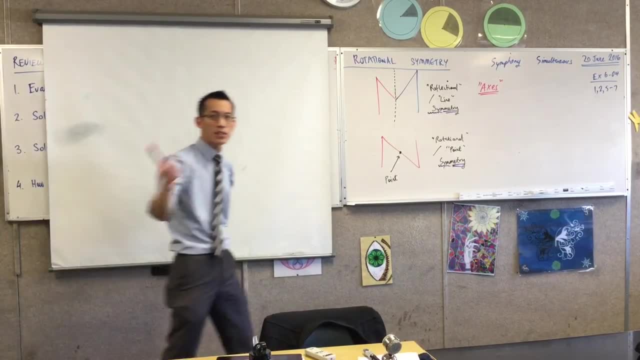 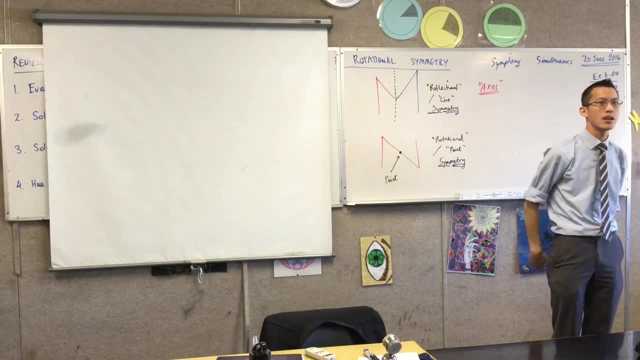 Okay, Objects you made last week. Right Now, have a look at some of them. Why do you have one? You'll notice the vast majority of them have one axis of symmetry- Right One axis. But in fact if you look at the one right next to Abby, that blue one, it's second from